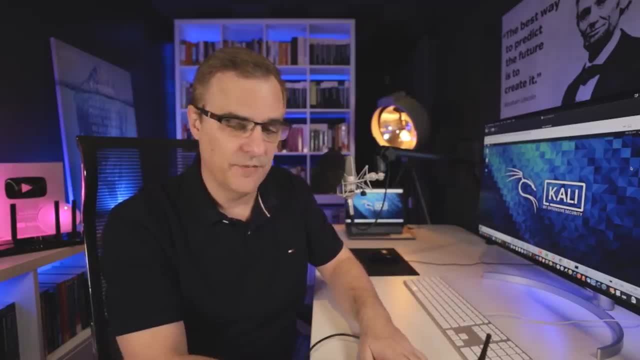 In this example, I'm using Kali Linux, or Kali Linux, if you prefer, within a virtual machine running on this Windows 10 laptop. Now you could run Kali natively if you preferred, but in this example, I'm simply running it within a virtual machine on Windows. 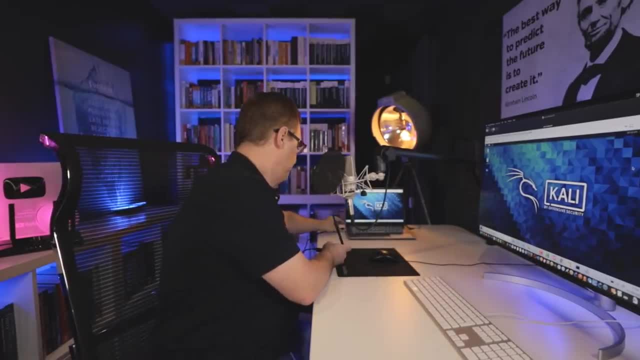 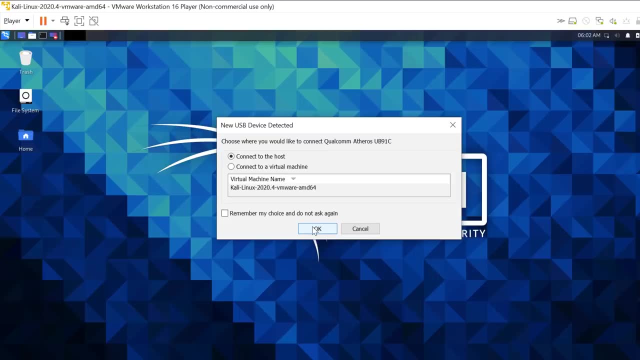 First thing you need to do is plug in the Wi-Fi network adapter. Okay, so now that it's plugged in, I'm asked by VMware: where do I wanna connect it? In my example, I wanna connect it to the Kali virtual machine. 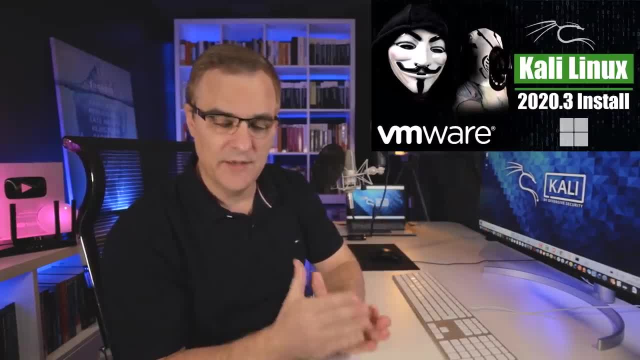 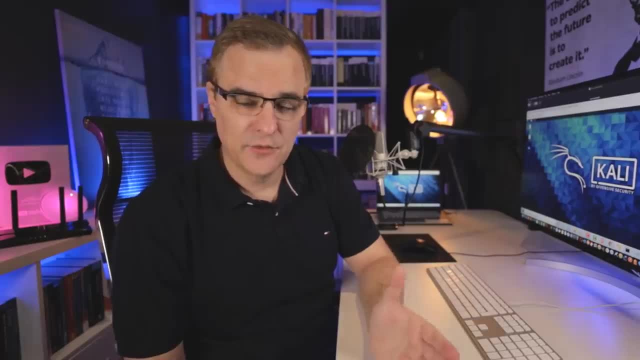 Now, in a separate video, which I've linked here and below, I showed you how to get Kali up and running within VMware Player. That's what I'm using here. So if you don't have Kali Linux installed and running, 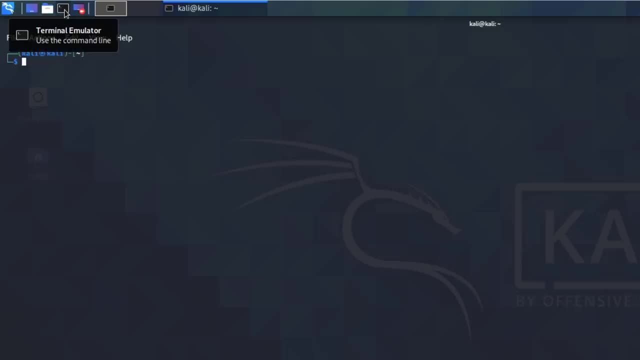 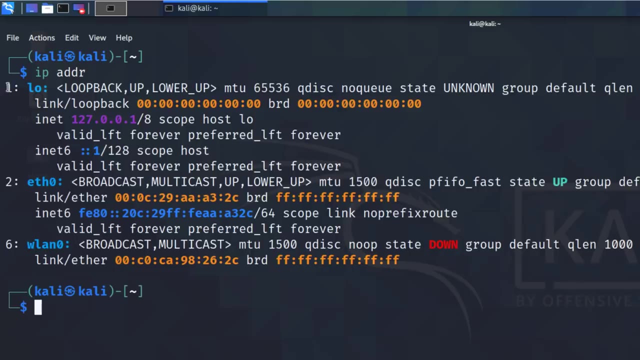 then have a look at that video. Now that the network adapter is plugged in, I'm gonna open up a terminal window and I'm gonna use a command IP address to see IP addresses and interfaces on this virtual machine. This is what we wanna see. 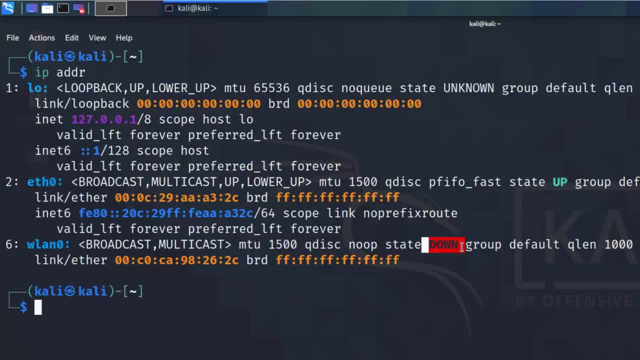 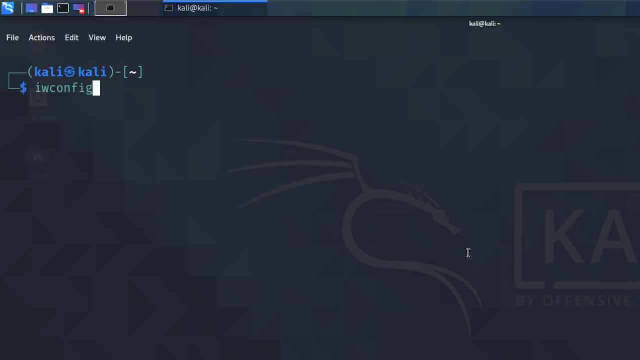 We've got a wireless LAN adapter. At the moment the state is down, but it's important that we see a Wi-Fi network adapter. You can also use the command iwconfig if you prefer, and that shows us that we have a Wi-Fi network adapter. 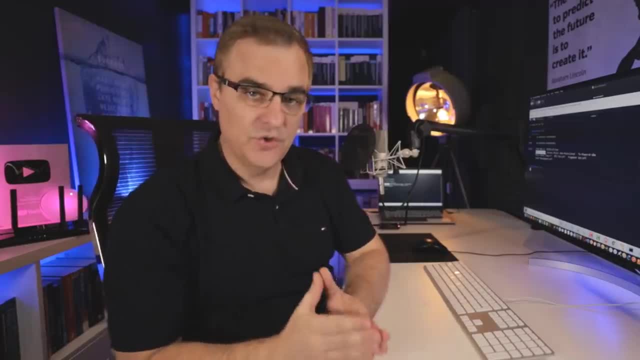 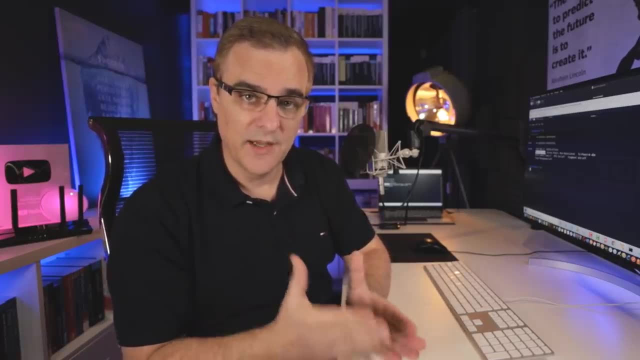 At the moment the mode is managed. We're gonna change that to monitor mode in a moment. but the first thing you wanna make sure is that you've got a Wi-Fi network adapter that's recognized by Kali. Next thing we need is a Wi-Fi network to attack. 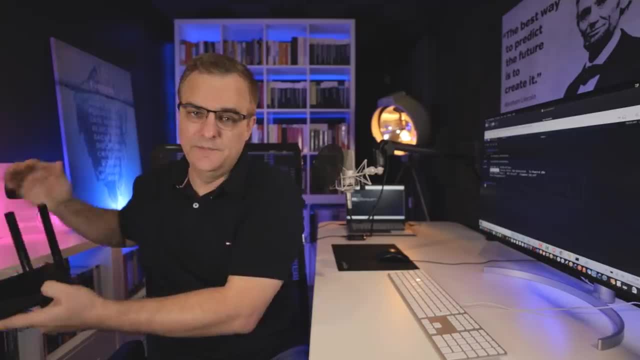 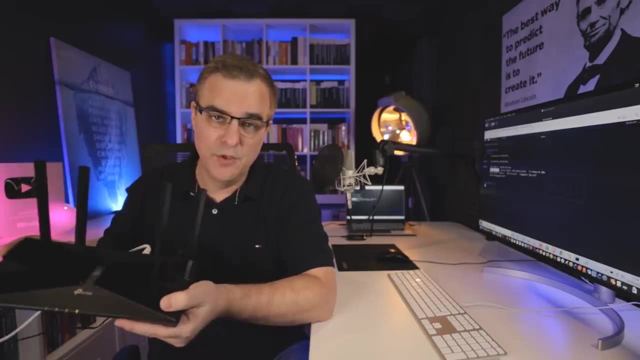 So for this demonstration, I've got a TP-Link router, which I've purchased. This is a TP-Link router that I'm gonna use simply for demonstration purposes, So this is a network adapter. This is a network that I own. 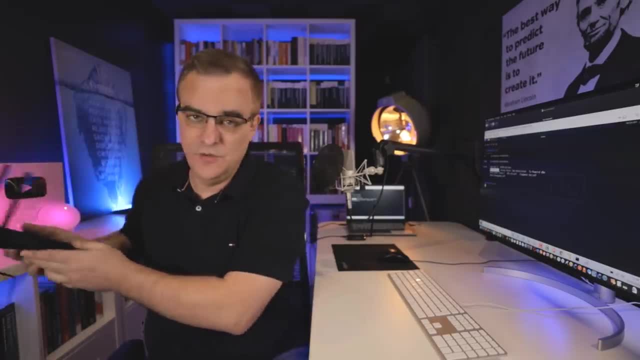 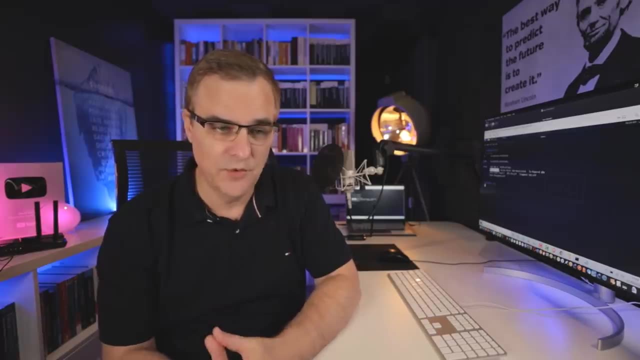 I'm not attacking someone else's network. Please do not use the information that I'm sharing in this video for nonethical purposes. What I'm sharing here is for educational purposes only. I have to say this, otherwise I get into trouble, so please bear with me. 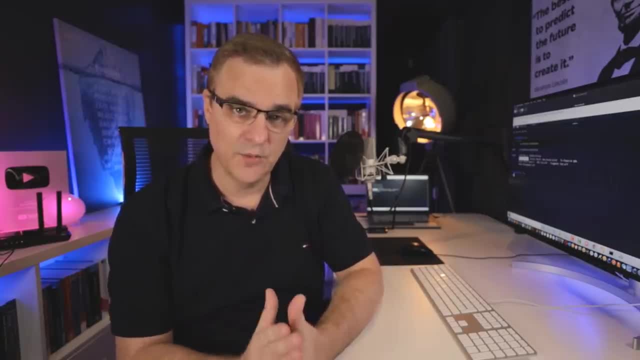 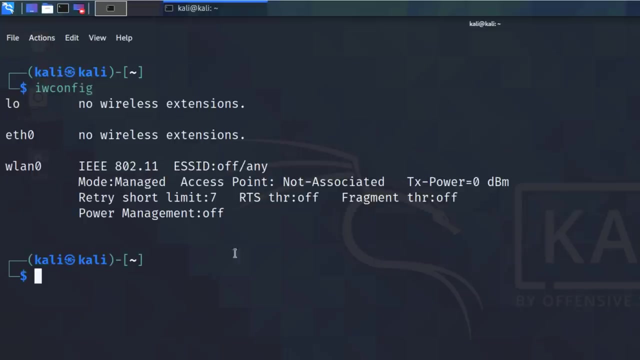 Only use this for ethical hacking purposes. Only attack networks that you own or have permission to attack. Once again, I'm attacking my own network here for demonstration and educational purposes only, Okay. Once again, iwconfig shows us that a Wi-Fi adapter is connected. 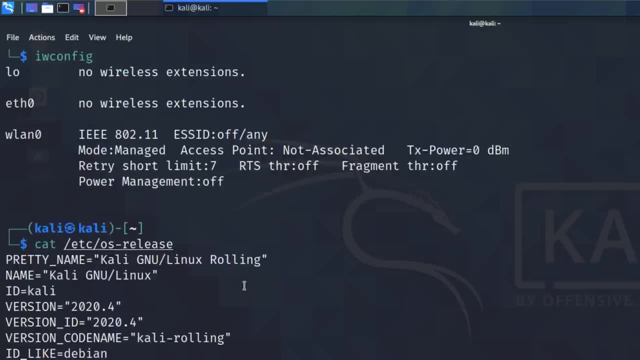 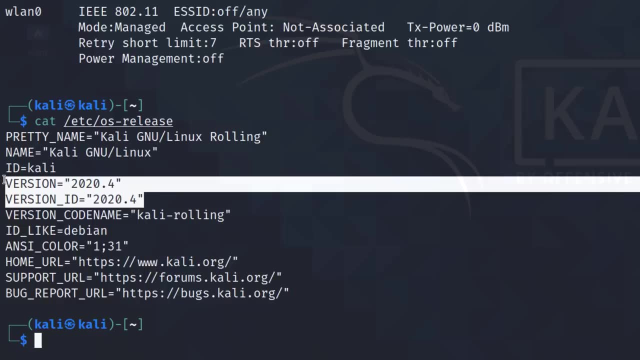 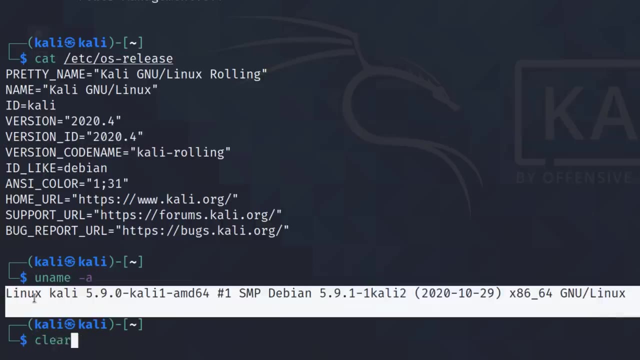 What I will show you here is I do have this release of Kali. So cat etsy os-release shows me that I'm using Kali 2020.04.. You could also use uname-a to see details of the Linux version. So once again, I'm using Kali in this example. 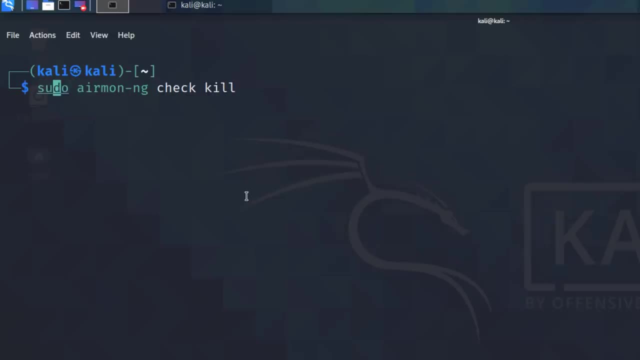 Okay, so the next step is to run sudo. That gives us root privileges. We're gonna use m on ng to check for any conflicting processes and kill them. We can see that this process was killed. Now in your example you may see a whole bunch. 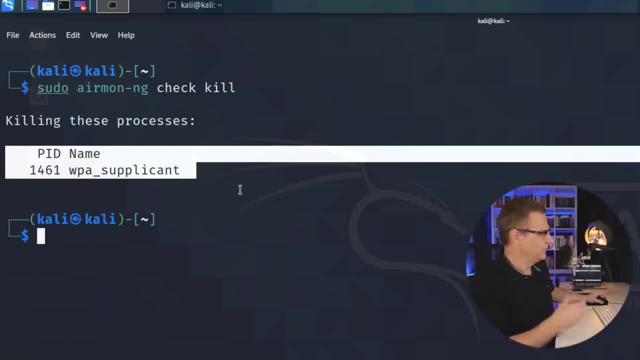 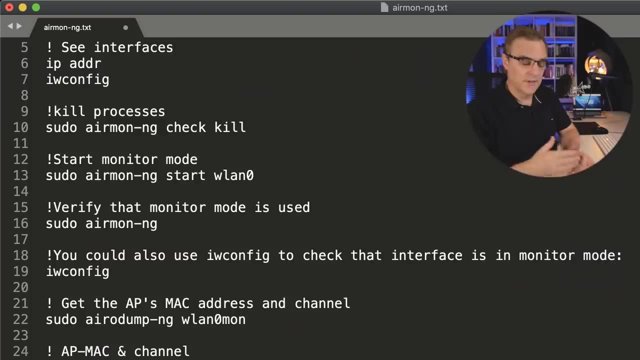 of other processes that get discovered and get killed, and that's fine. Just make sure that you type this command so that you don't have any conflicting processes that interfere with what we're trying to do Now to make this easier for you. 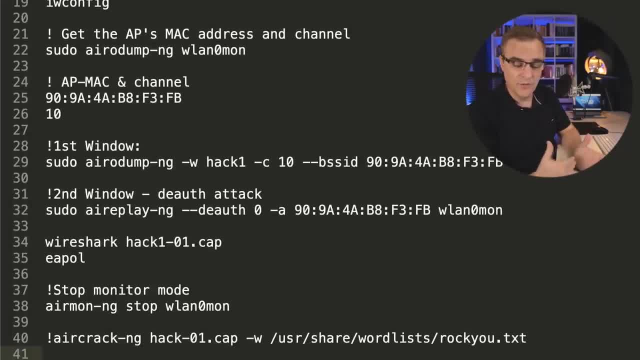 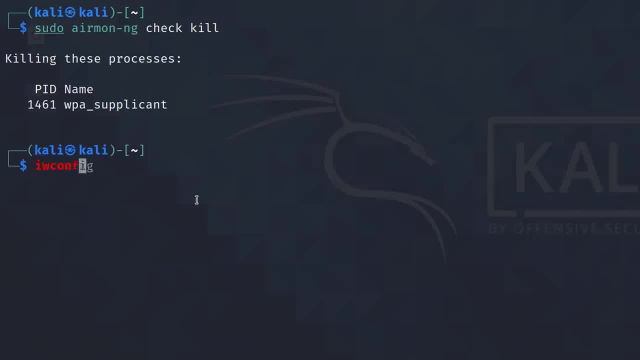 I've put all the commands below this video. So if you wanna follow along with what I'm doing, then please watch the full video. But if you need the commands as a reference, I've put them below. Okay, so once again, iwconfig shows us. 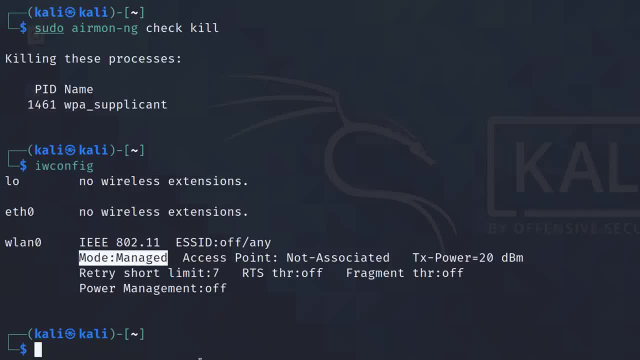 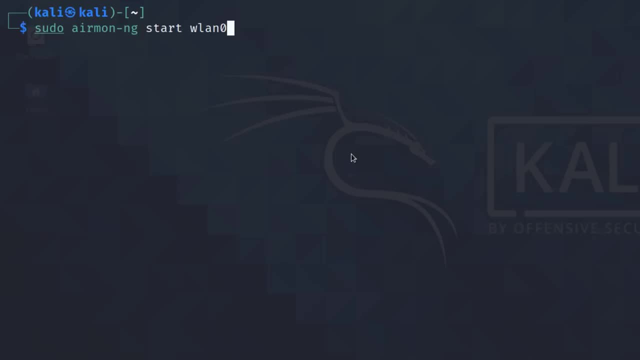 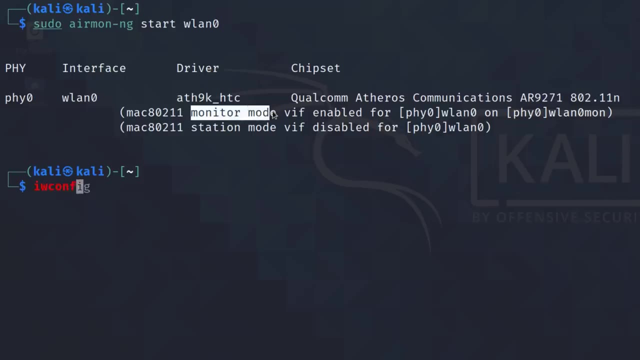 that the wireless network interface is in managed mode, but what we wanna do is put it into monitor mode by using the command sudo m on ng start wlan0.. We can see that monitor mode is now enabled. Iwconfig shows us that the mode has been enabled. 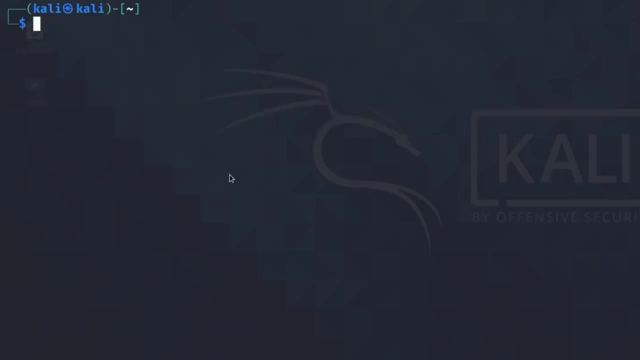 The mode has changed from managed mode to monitor mode. You can also confirm that by using the command sudo m on ng. Notice the wireless interface is now wlan0 mon. Before it was wlan0, but now it's changed to wlan0 mon. 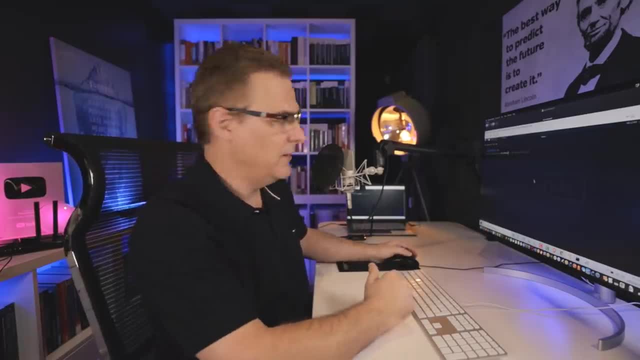 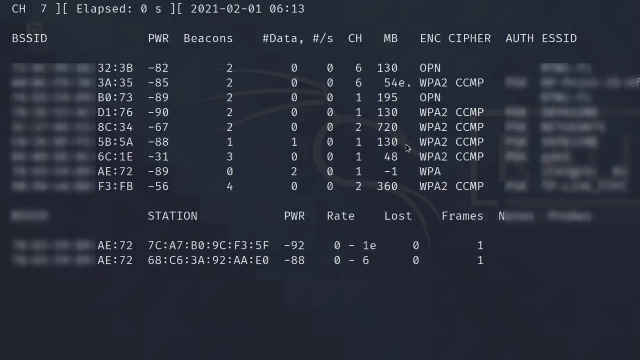 Okay, so now let's discover the access points, and hopefully I'll discover that access point behind me. To do that, we use the command sudo, erodump ng wlan0 mon And, as you can see, a whole bunch of wireless networks are discovered. 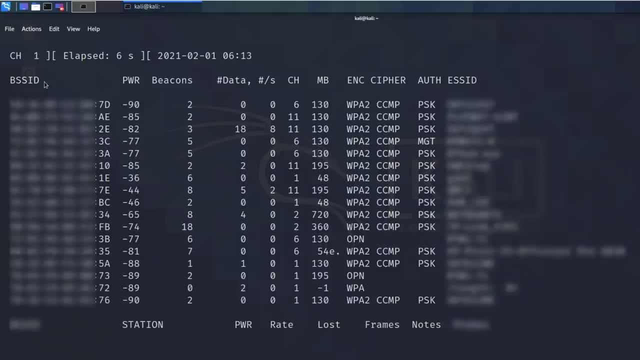 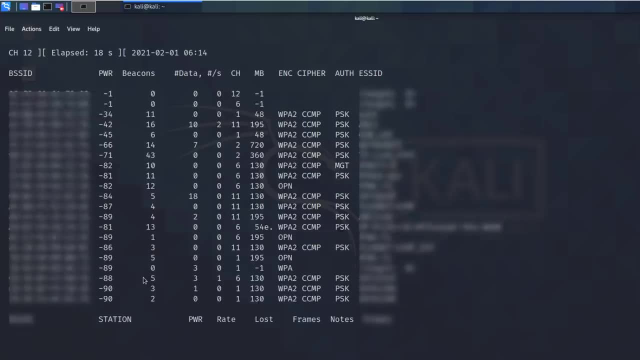 So here are the various SSIDs or MAC addresses of the wireless networks. I'll make this a little bit smaller And, as you can see at the bottom here, various stations have been discovered. I've made the font really small. I'll press Control C to cancel that. 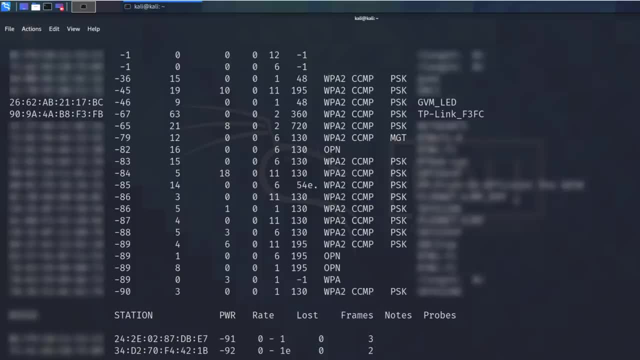 So Control C to break and I'll zoom in. The network that I'm interested in is this network, TP-Link F3FC, And I'm gonna go ahead and click on that. TP-Link F3FC Notice it's using channel two. 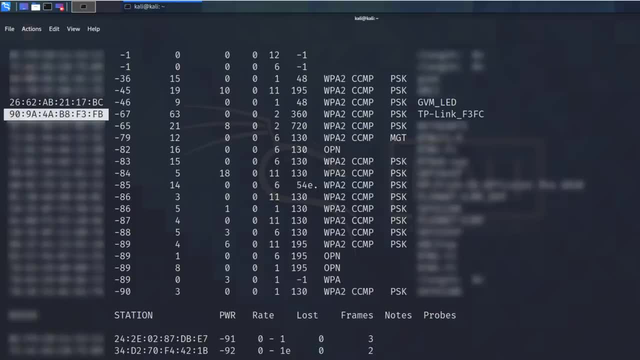 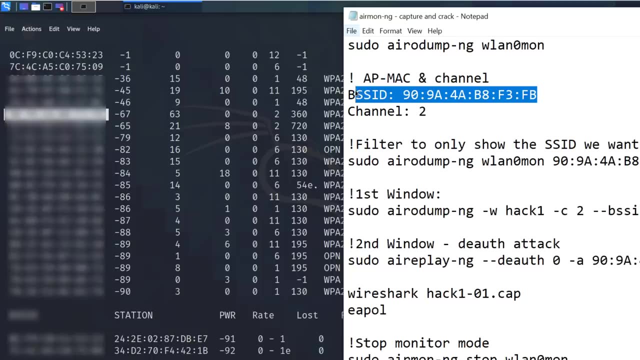 and that's the MAC address of the access point. So you're gonna wanna take a note of that. I've added that information to my script. So channel is two BSSID. is that Scrolling up? we can see once again. 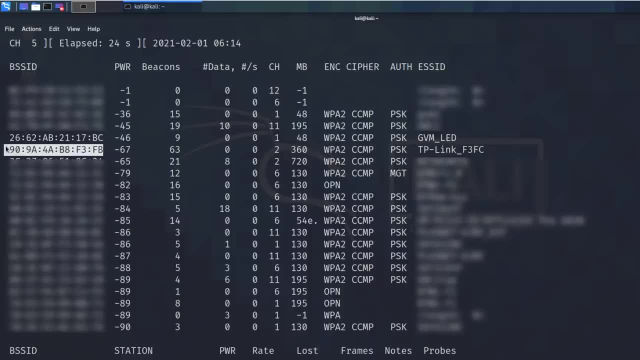 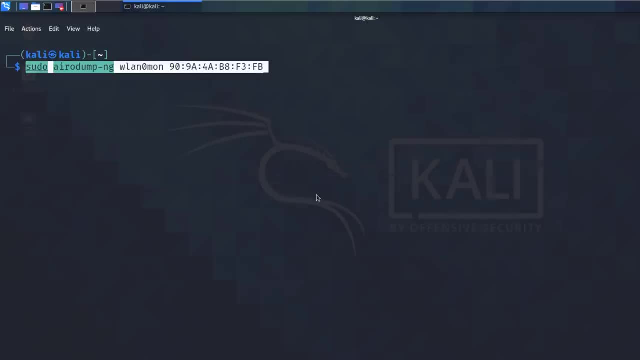 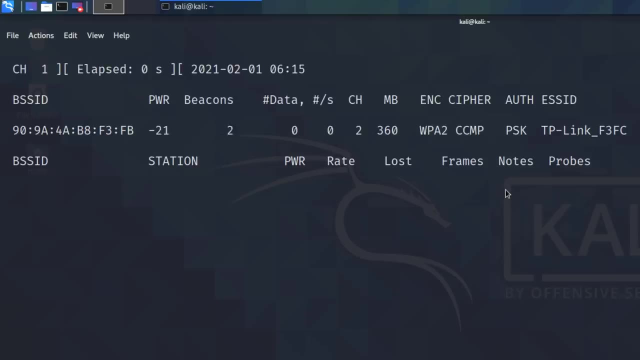 channel is two for this access point MAC address is that? I'll clear the screen And what you could do is use the command sudo erodump ng dash D and the MAC address to display only that access point, So we can see the BSSID. 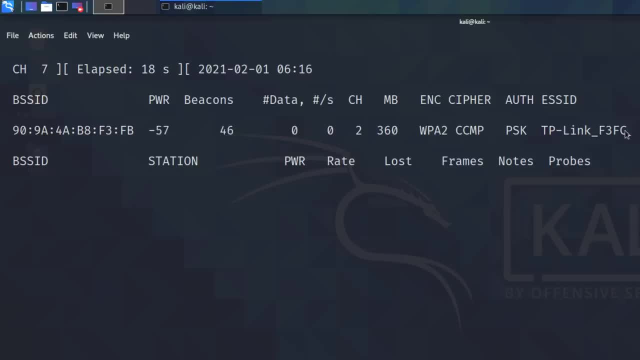 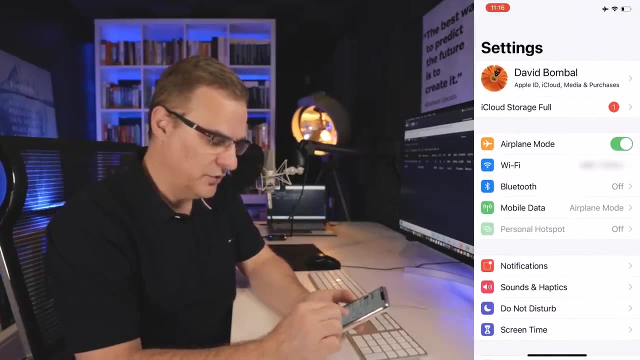 We can see how many beacons are being sent. We can see the ESSID or the name that we as a human would use. Now I could use a phone as an example to connect to that network, So I'll connect to that network. 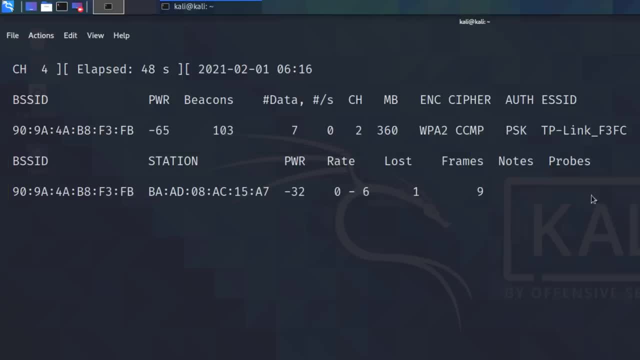 And hopefully what we'll see is that a client has connected. And there you go: We can see that this client has connected to that network. Okay, so I'm gonna cancel that And we're gonna use the command sudo erodump ng dash W. 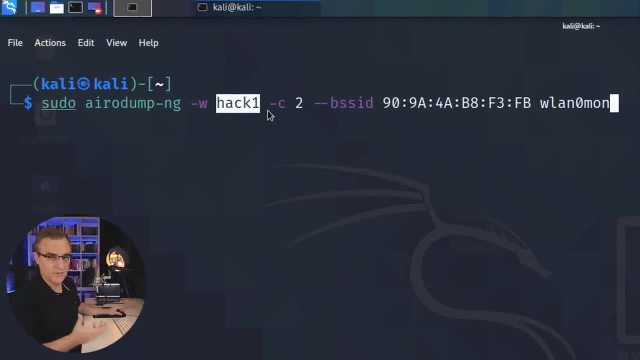 This is the name of the file that we're gonna store the captures in. So I'm gonna store the CAP file as an example to open with Wireshark in a file called hack one. The channel that we're gonna attack is two. The BSSID that we're gonna attack is this: 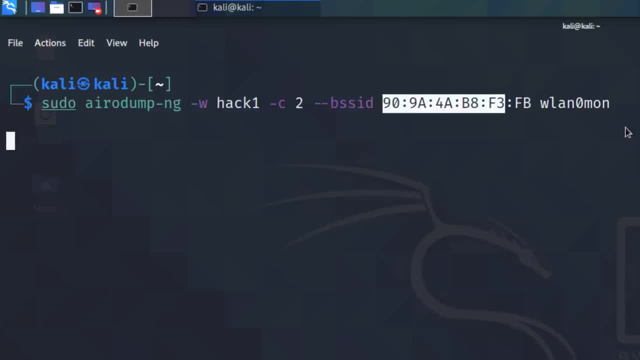 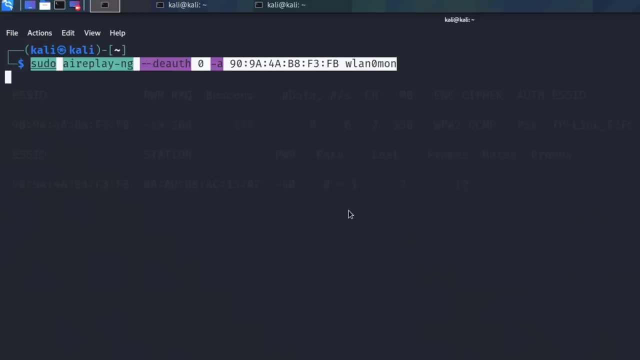 And the interface we're gonna use is wlan0mon. So in one window open that up And then in a second window deauthenticate clients from the network. So just before I press enter at the moment, notice we haven't got anything displayed here. 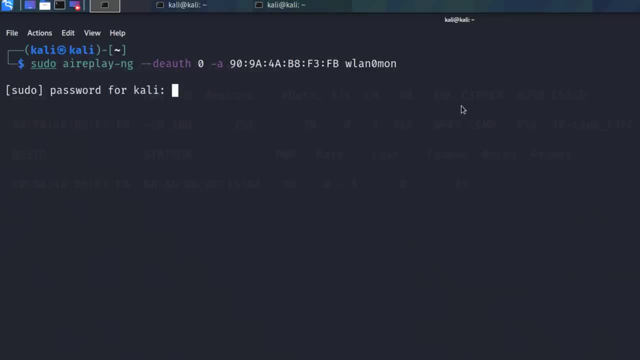 We haven't captured the four-way handshake. But as soon as I deauthenticate clients- and this deauth0 means we're not gonna stop the number of deauthentications used against that access point Notice- a whole bunch of deauths are sent. 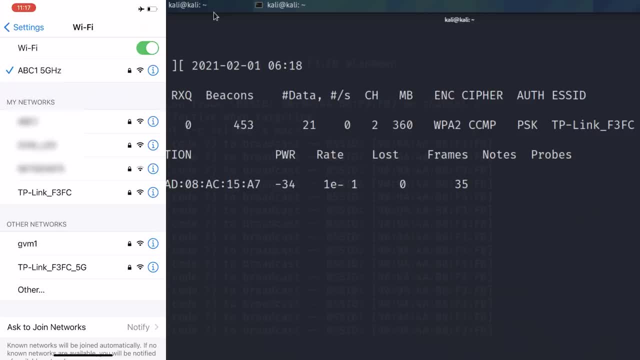 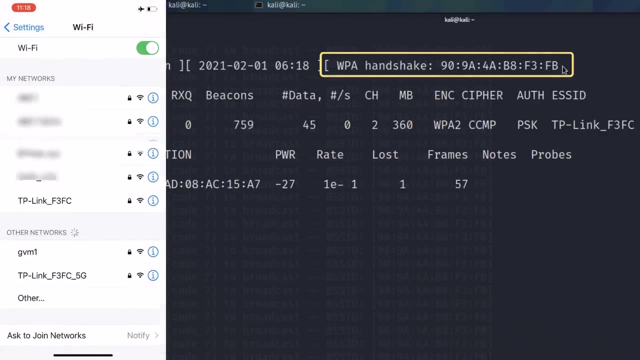 On my phone. it's moved from one access point to the other. I'll try and connect back to the TP-Link network And hopefully what we should see is that a four-way handshake is captured. Okay, so there you go. You can see the WPA handshake was captured. 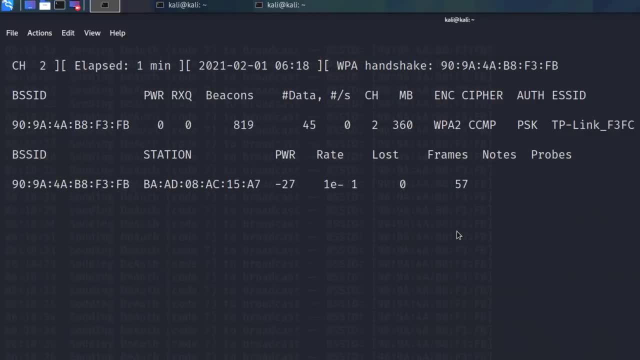 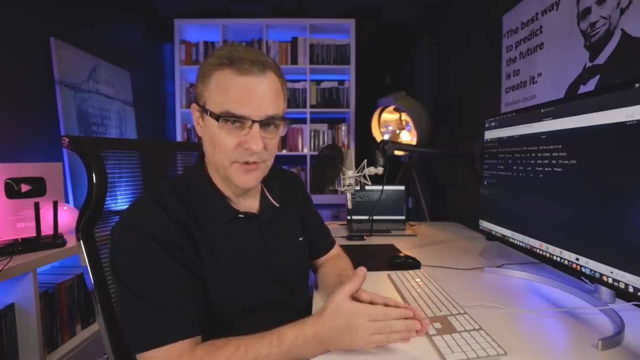 Client is not able to connect to the network, but we captured the handshake. Control C allows me to stop this process, So you could simply use that script as an example to deauthenticate everyone off a network if you wanted to. So that's another attack. 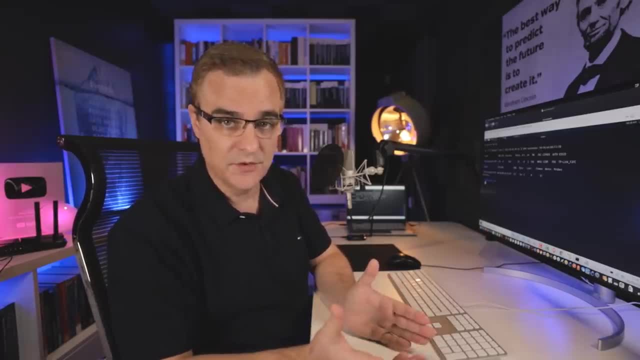 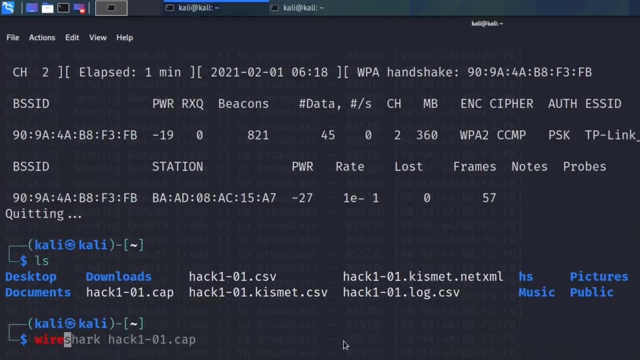 You could do a denial of service attack against an access point just to stop anyone connecting to it. But in this example, if I type LS, what you'll notice is we've got this hack file captured And what I could do now is use Wireshark. 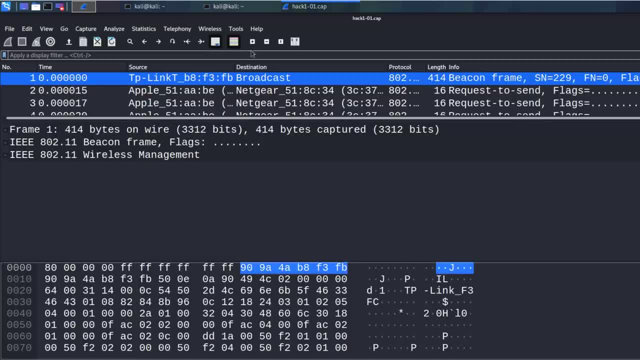 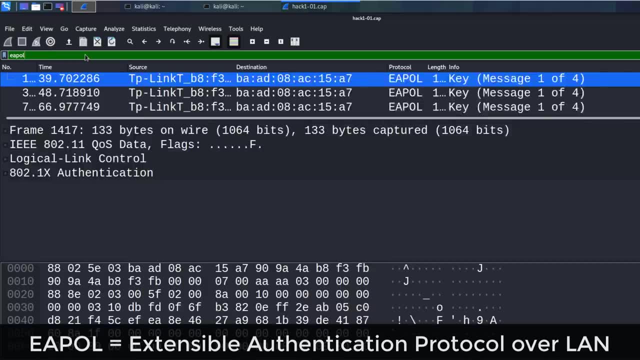 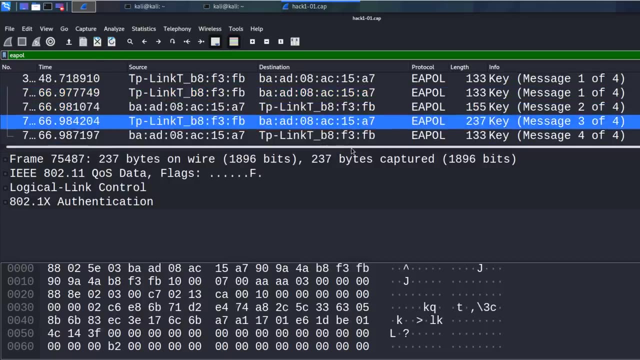 to open up that cap file. So a whole bunch of information has been captured, but I'm gonna search for the handshake And notice. here you can see message one, message two, message three, message four. So we've captured the WPA four-way handshake. 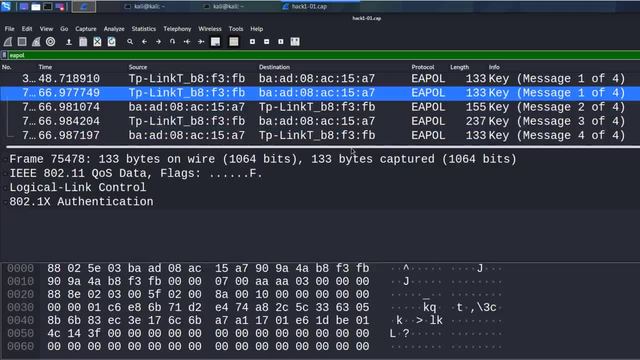 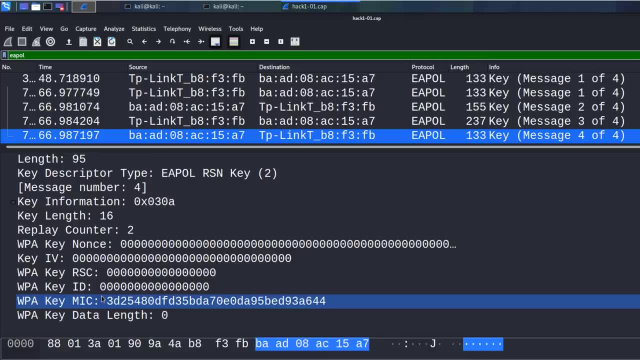 We had some additional messages, but here's the full four-way handshake between a TP-Link device and my iPhone So you could open up the Wireshark capture and have a look. but notice, in message two we see WPA key data sent from the iPhone. 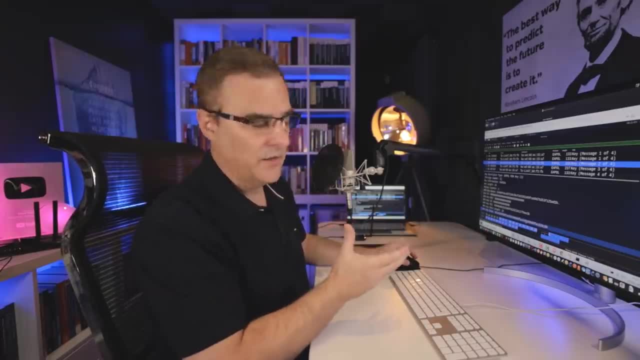 to the TP-Link access point, And that's what we wanna crack. So the iPhone is sending authentication communication information to the access point. We're capturing that and that's what we're going to decrypt. Okay, so I'll close that down. 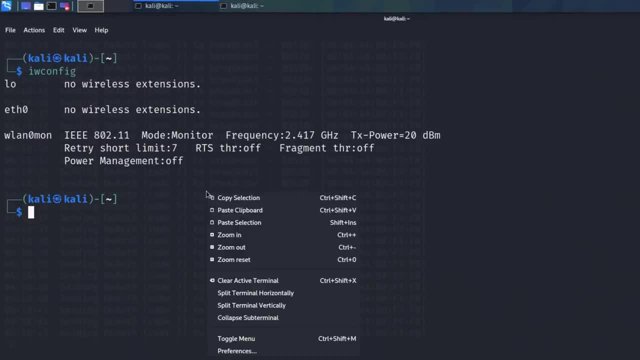 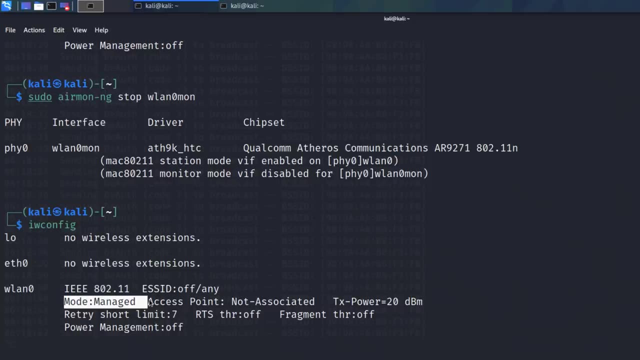 At the moment the Wi-Fi interface is still in monitor mode, So what I'll do is stop monitor mode. IW config shows me that the interface is back in managed mode. Be aware that when you put an interface into monitor mode it'll break your internet connection. 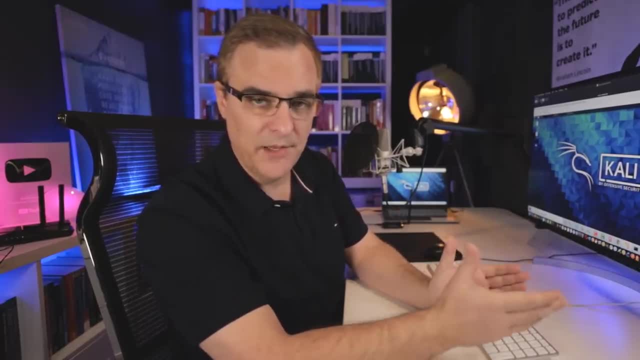 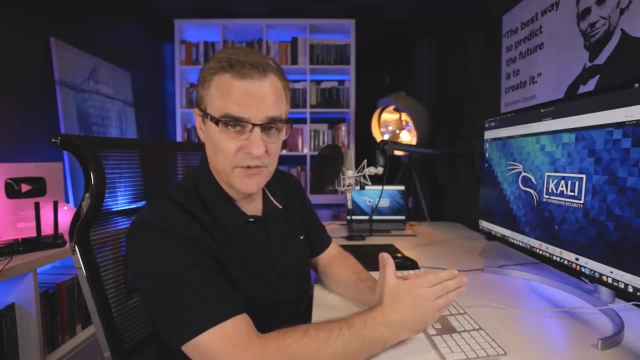 You won't be able to use that interface for connections onto the internet or other places, because it's monitoring traffic. Another reason to use a VM preps is in this example: I've got two network adapters The Kali Linux virtual machine is actually using. 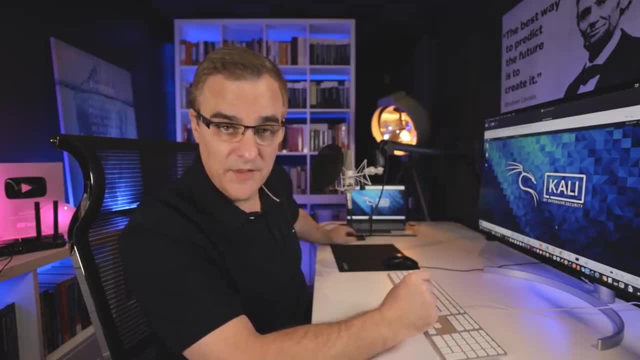 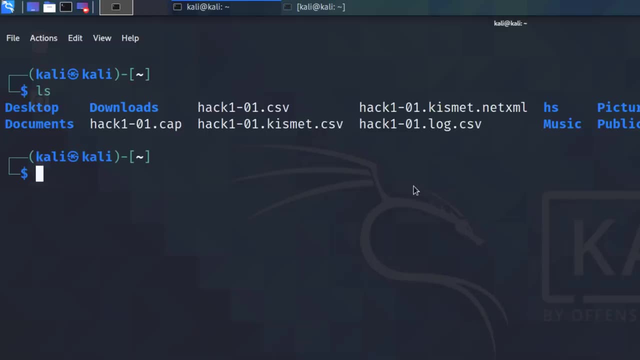 the Wi-Fi adapter of Windows to give it internet connectivity, but the external alpha adapter is in monitor mode. Okay, so let's clear the screen. So Alice once again shows me the files. Hack01cap is the file that we wanna use for cracking. 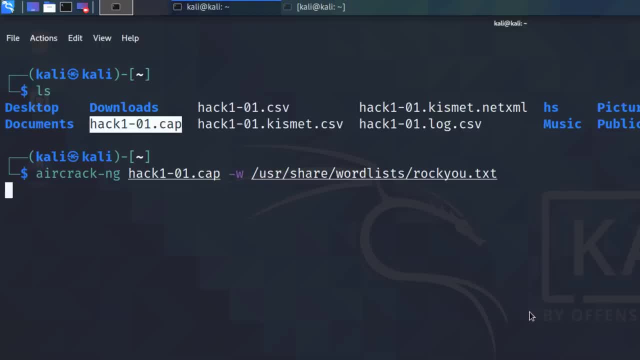 And to do that we're gonna use this command aircrackng. So I'm gonna go to Kali hack01cap and the word list that I'm gonna use is stored in user-share-wordlist-rocku. So just to show you what that is: 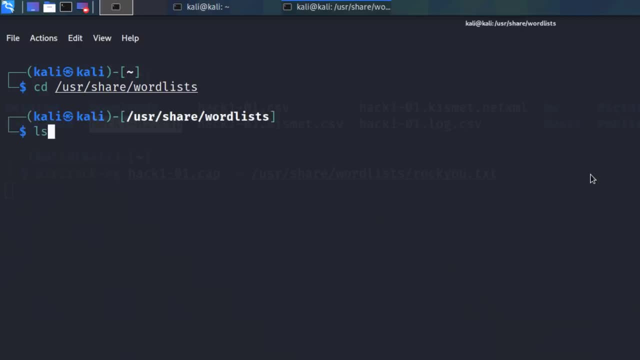 if I go to user-share-wordlists, various word lists are stored in this directory In Kali. you can actually just search for word lists and it will show you the various word lists available in Kali, And one of those is the rocku file. 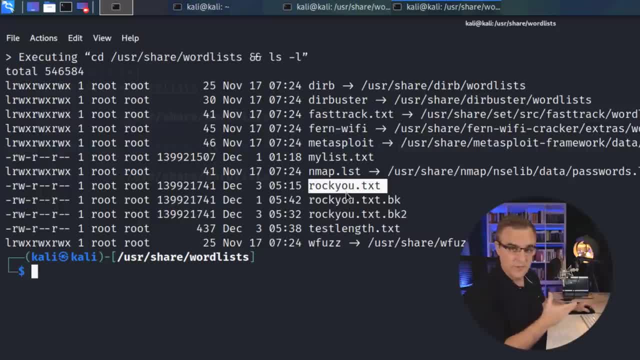 Now it needs to be unzipped so you can use gzip to unzip it, and that's what I've done here. I showed you how to do that in this video, so have a look at that video if you wanna see how to unzip the file. 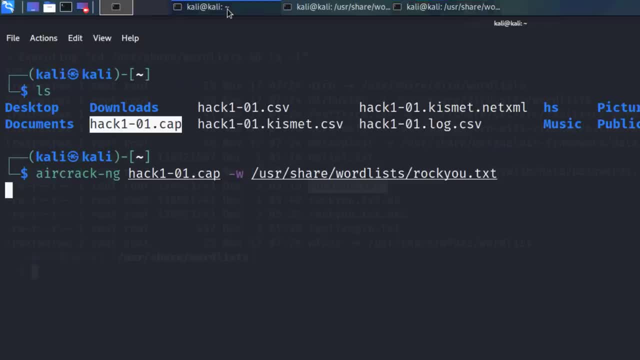 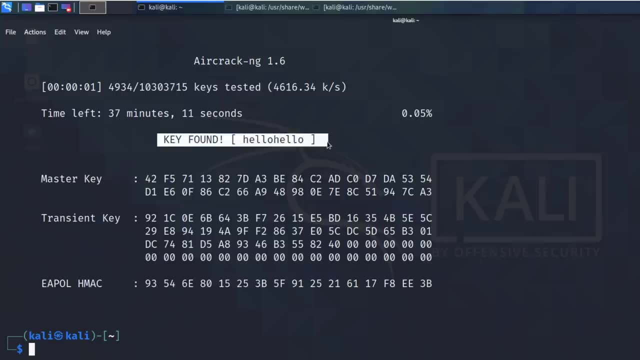 and use that word list, But that's the word list that I'm gonna use, So let's try and crack that password with the word list. And there it is. The password that I used was hello- hello. Now you might say: 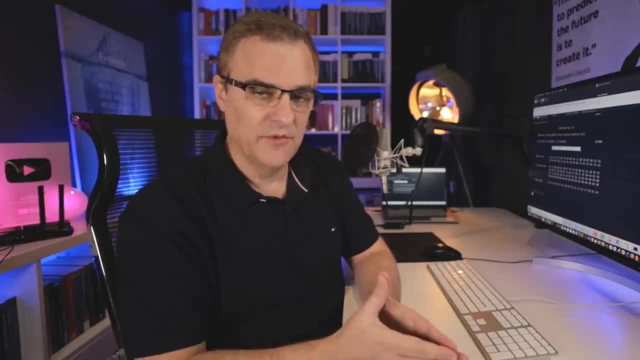 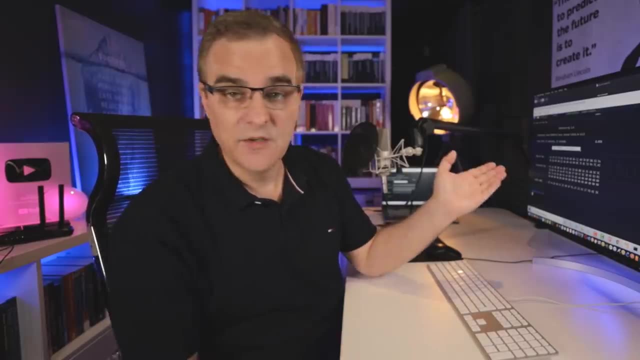 well, David, that password is too simple. This is just for demonstration purposes. The rocku word list has millions of passwords in it, actual passwords used by people. So what I did is just find a password in that word list and I configured this TP-Link network with that password. 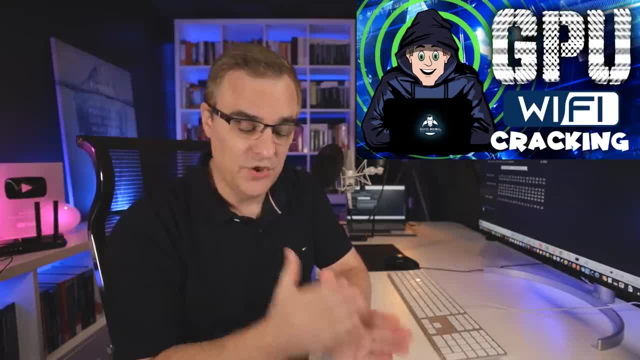 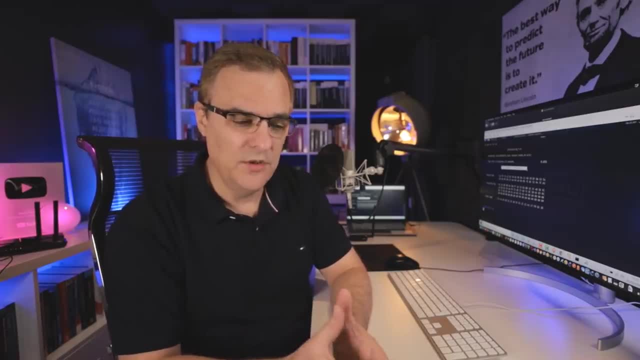 In separate videos such as this one, I showed you how to use a GPU to crack a non-standard password. I'll also create additional videos where I use a very powerful GPU to crack a WPA pre-shared keys that are non-standard passwords. 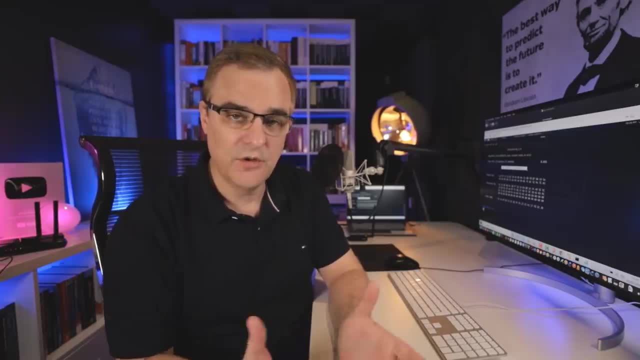 But in a lot of cases people use passwords stored in the rocku file, In the rocku word list. Just because people are supposed to do something doesn't mean that that's what they do. Hopefully you're using a much better password. 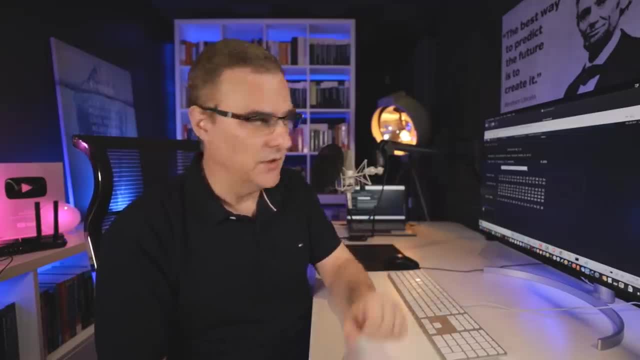 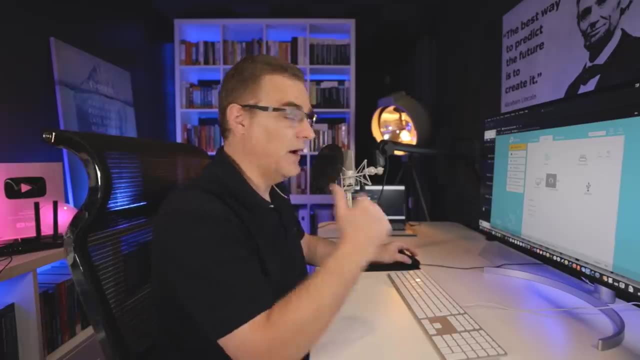 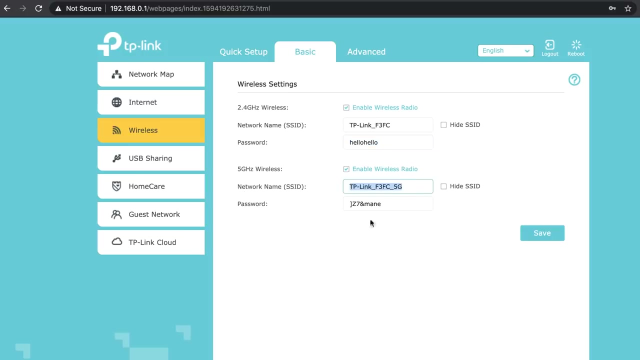 than something simple like this, But this is a password in the rocku word list. For this demonstration, I once again configured that TP-Link router behind me with this password, So you can see this network has this password. This is the password of the 5G network.